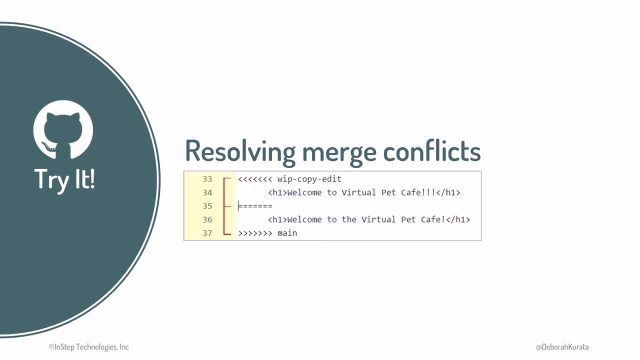 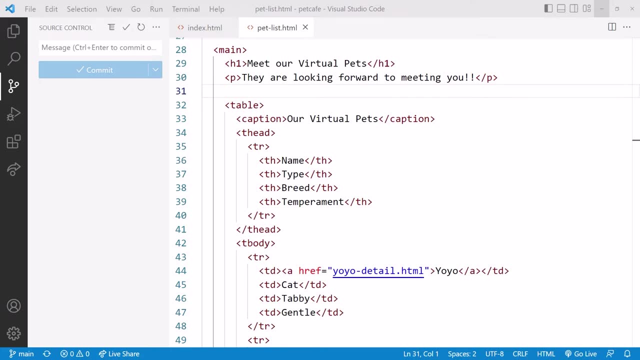 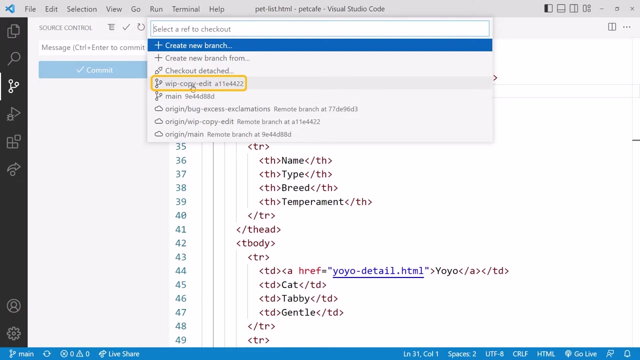 change to that same line to cause a merge conflict Back in VS Code. we'll work more on the whip-copy-edit task. First we need to ensure we are on the correct branch. Click on the branch down here And up here, switch to the whip-copy-edit branch. Git automatically changes the content. 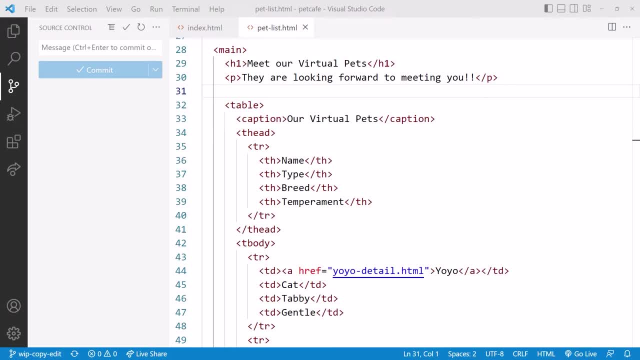 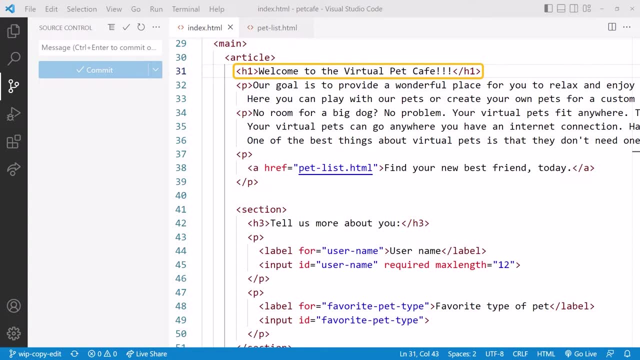 of our working folder to the last commit on that branch. Looking at the indexhtml file we see our extra exclamation marks again. Our fix to remove them in the merged branch didn't impact this branch. At this point we should merge the updated main branch into. 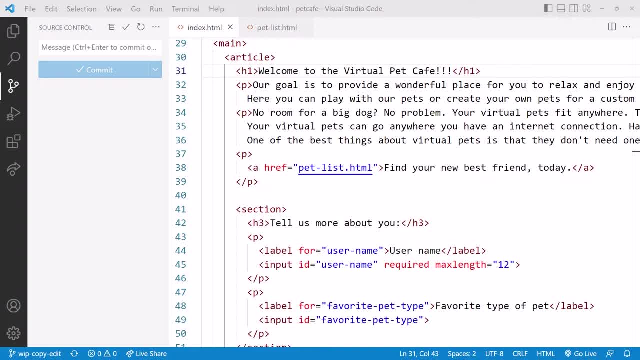 any remaining branches to prevent possible merge conflicts. But we want to see how to resolve merge conflicts, So instead we'll skip the merge now and change that same line to ensure we get a merge conflict. Let's remove the from the heading. You don't say welcome to the GitHub, so we shouldn't. 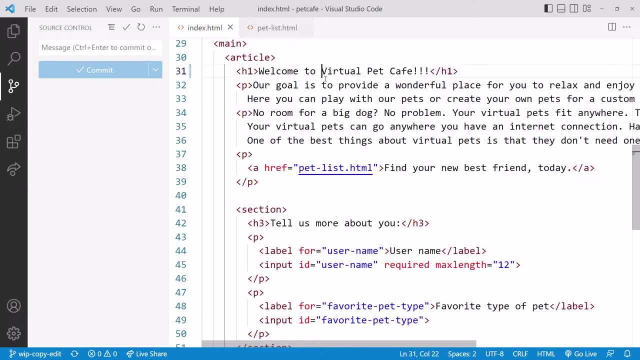 say welcome to the virtual pet cafe Done. We see in the source control panel that the indexhtml file has been removed. The indexhtml file has been removed. The indexhtml file was modified. Let's type in a commit message: Copy edits for index heading. Then click the. 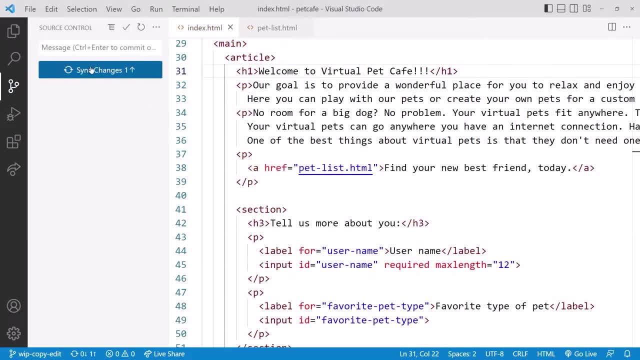 check to commit And confirm. Now we can click sync changes to push the change to GitHub. We'll double check the confirmation message to ensure we are committing to the correct branch. We are, so click OK, No problem so far. Let's say we finished our copy edits. 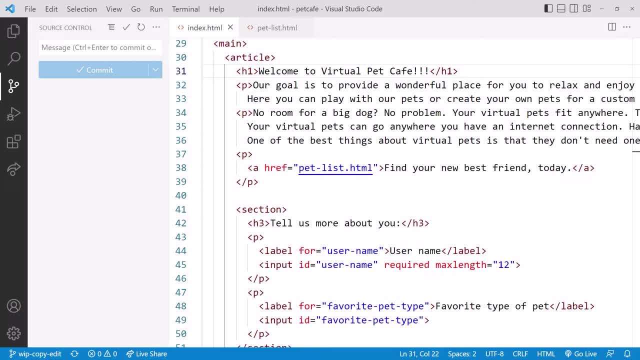 and committed our changes. We're now ready to go back to GitHub. Let's go back to GitHub. We're now ready to go back to GitHub. Let's go back to GitHub. Let's go back to GitHub. We're now ready to issue a PR. We do that on GitHub. Refresh the browser to see the 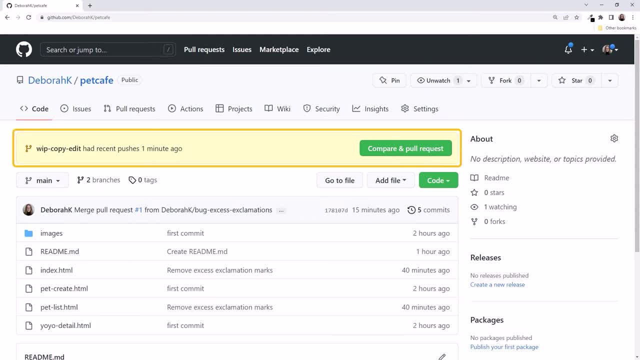 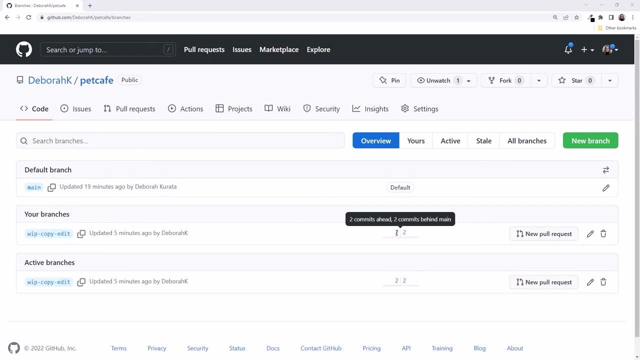 current changes. As we did last time, we could click the compare and pull request button here, But so we can see how to do it another way. let's click on branches and issue the pull request from there. We see that this branch is now two commits ahead our two copy. 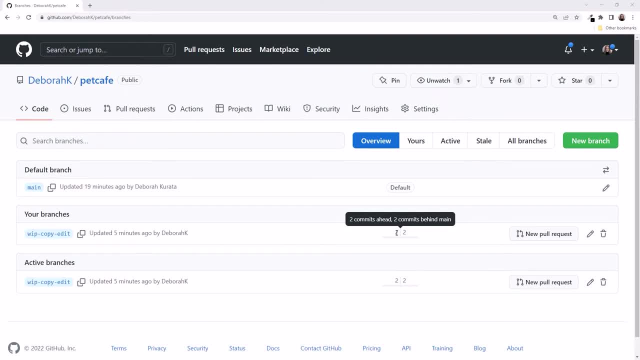 edit commits And it's two commits behind. These are the commits from the bug-excess-exclamations branch. we merged into main but not into this branch. Let's click new pull request to open a new pull request. It provides a default. 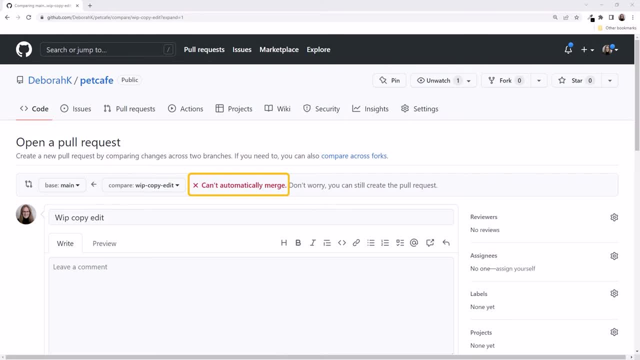 title we can edit as desired. Notice the message here. It's already telling us that it can't automatically merge for us. We have a conflict, But it's so reassuring telling us we can still create the pull request. Scroll down to the top of the page. We can see that we. 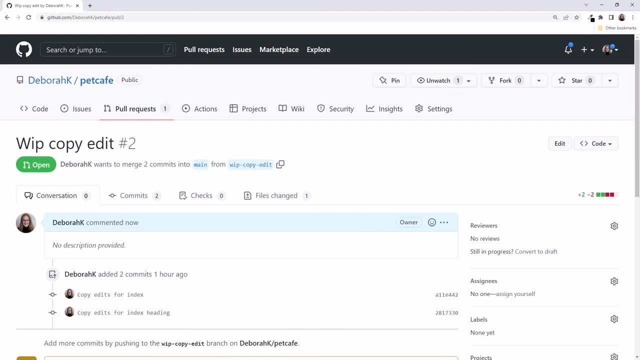 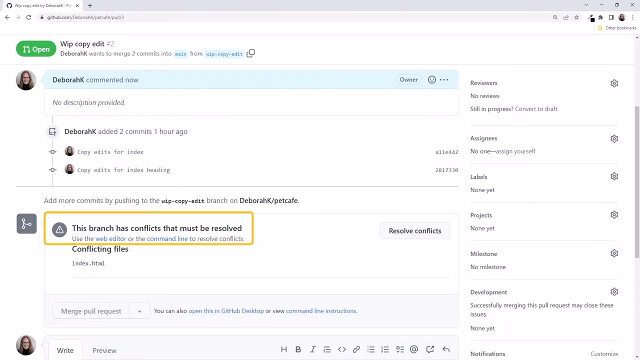 can now pull the pull request down And click Create pull request. Here's the pull request. Scrolling down the pull request notifies us that the branch has conflicts that must be resolved. It even tells us which files have the conflict. Lucky for us in this case. 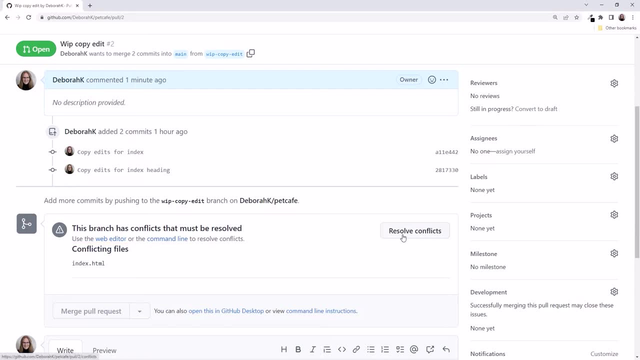 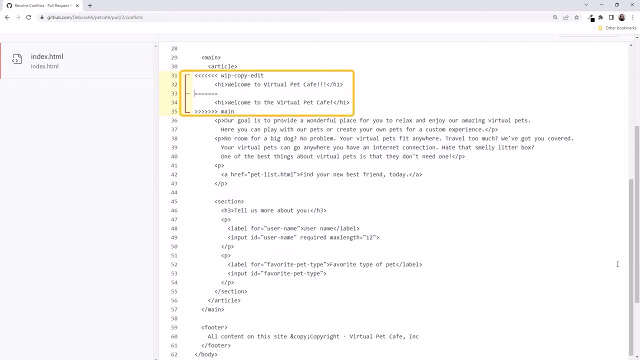 it's only one Click resolve conflicts to open the built-in editor and see the conflicts Scrolling. we see the conflict is right where we were expecting it. selecting Git adds conflict resolution markers to point out where the conflict occurs. The content above the equal signs is the content from our branch. 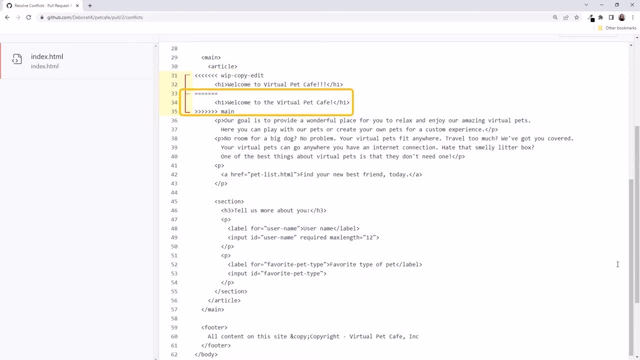 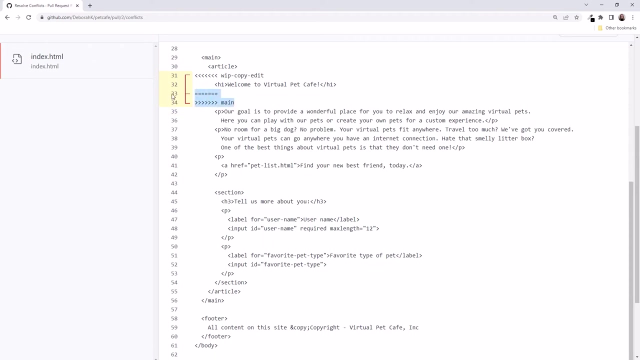 Below the equal signs is the content from the main branch. Now we have a chance to look at both changes and decide what to do. Let's start with our copy edit branch and remove the extra exclamation marks. Then we delete the duplicate text and delete the markers. 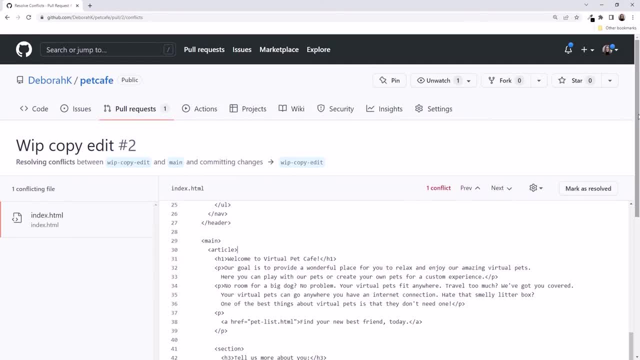 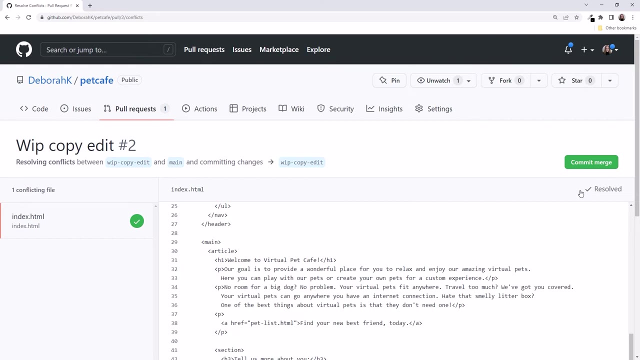 Using the outer scroll bar. if there were multiple conflicts, we'd use these buttons to navigate through them. When all of the conflicts are resolved, click Mark as Resolved. Our merge resolution caused a change to our copy edit branch, so GitHub commits the change. 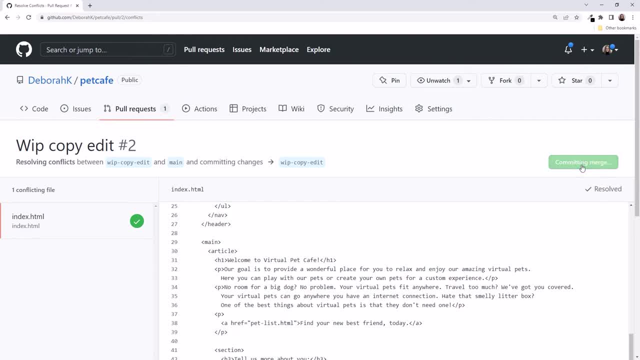 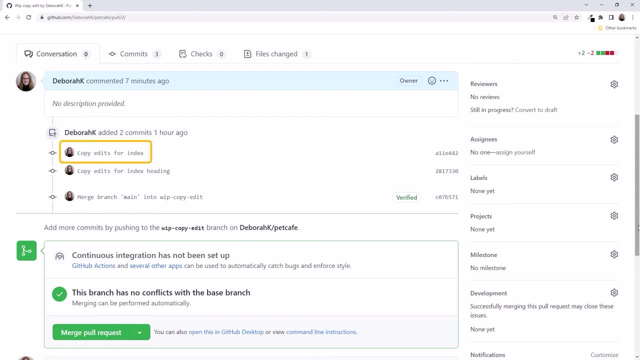 to that branch, Click Commit Merge to continue. Notice that we now have an additional commit in our branch. The first commit was for the first copy: edit- change to the indexhtml file. We changed some text to plural form. The second commit changed the heading removing the word the. 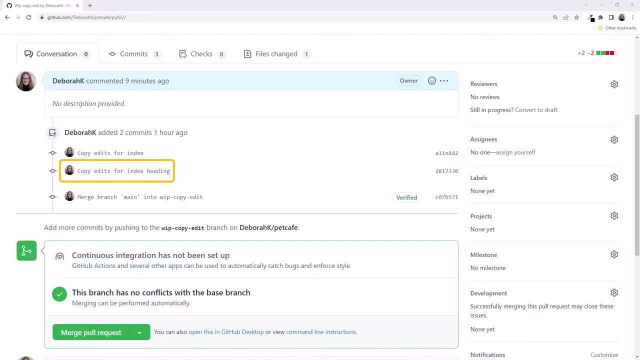 Since we'd also changed this heading in our bug-excess-exclamations branch, this change generated our merge conflict. This third commit was from resolving the conflict. Before we merge the PR, it's a good idea to check the files changed here to ensure. 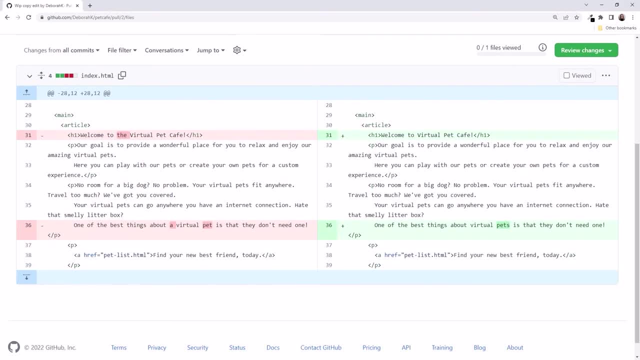 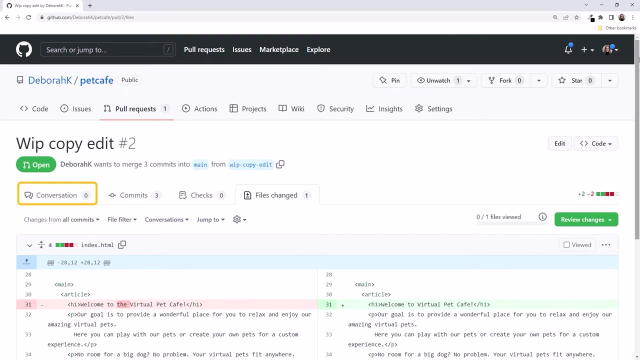 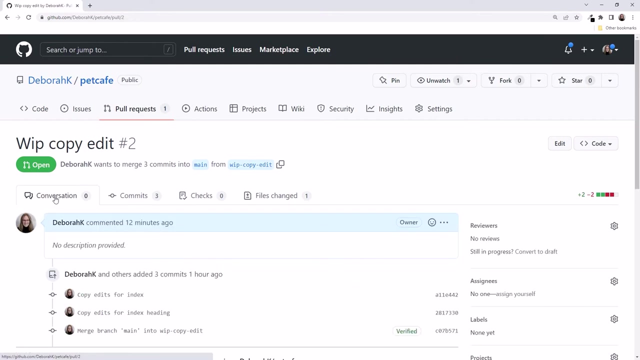 the changes match what we were expecting. These are the right changes, so we're good. Scroll up. Click Conversation to go back. Note that this is different from Conversations here. Now we're ready to merge the PR Scrolling down. 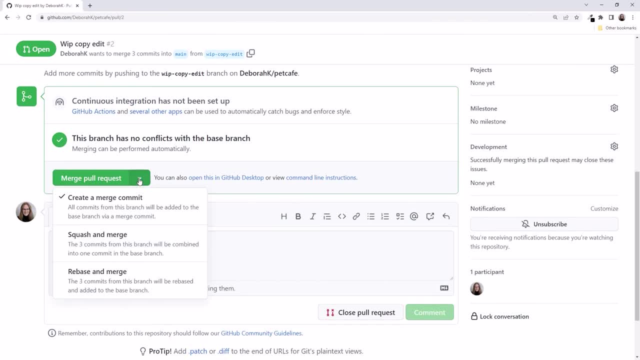 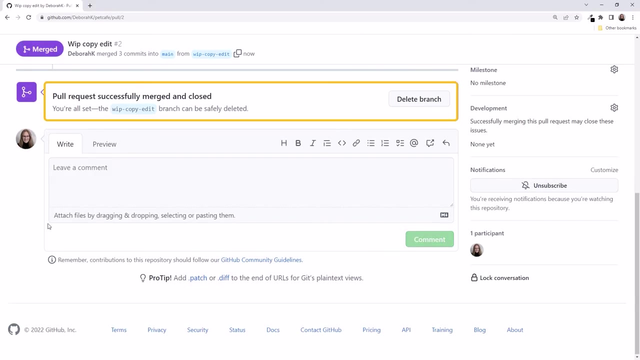 As before, we have options for how we do the merge. Because we now have three commits on this branch, we'll select to squash them and merge in one commit to the main branch, Then click the button and confirm Our pull request was successfully merged and closed. 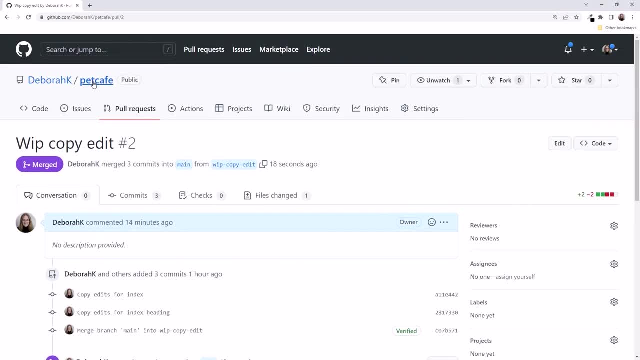 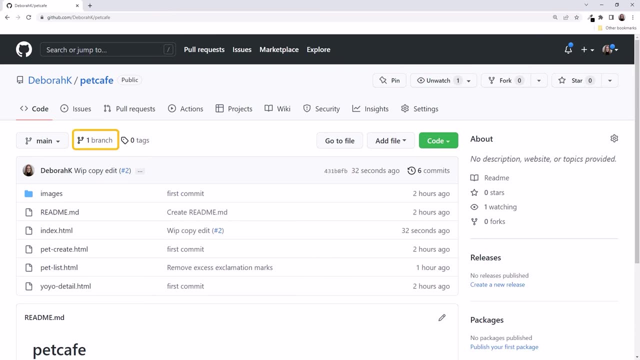 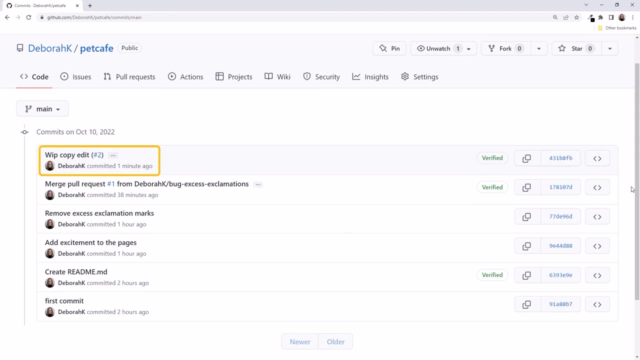 Now let's delete the branch. Scroll up And to go back we click the repository name. We now only have one branch, our main branch. Click on the commits to view the commit history And we see only one commit from the copyedit branch. 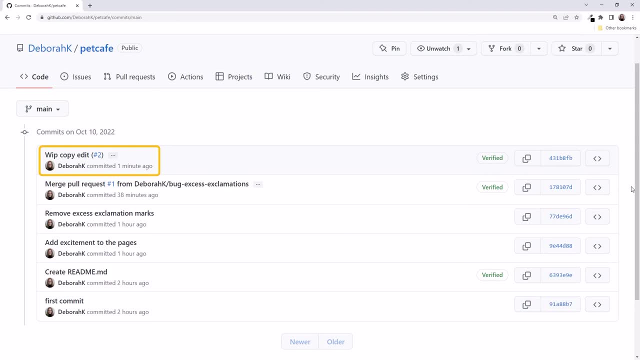 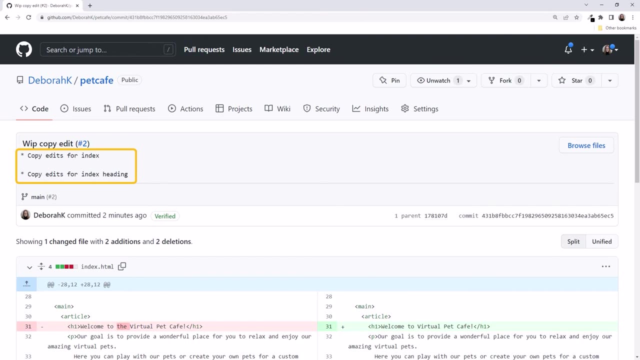 That's because we squashed the branch's commit history into one commit. Click on the commit name to view the commit details. We see here our original commit messages providing the details of what happened and retaining the branch history. Cool, We'll again click the repository name to return to the main repository page. 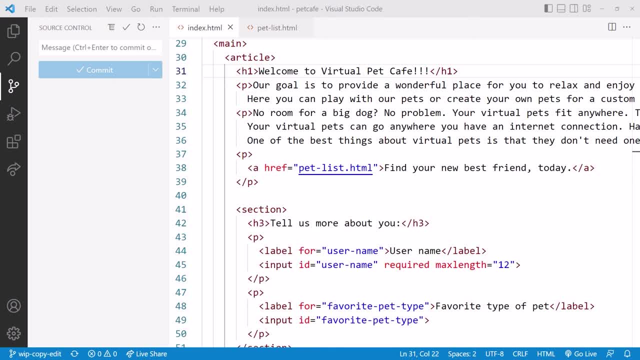 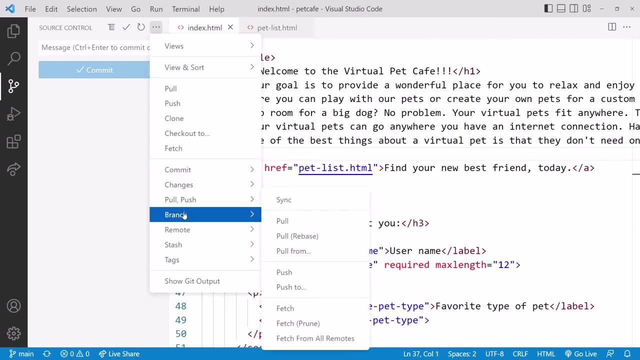 Cool, Back to VS Code. we want to delete our local WIP-COPY-EDIT branch. Recall from last time that we can't delete a branch we are on. so we'll start by switching to our local main branch. Then use the three dots here and select branch. 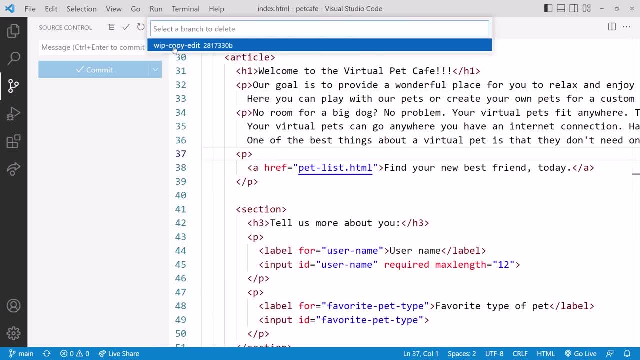 Delete branch. Pick to delete the WIP-COPY-EDIT branch. Now that we are back on the main branch, look at the indexhtml file. We still see the exclamation marks. Why is that? All of our merge conflict work hasn't been reflected yet in our local repository.